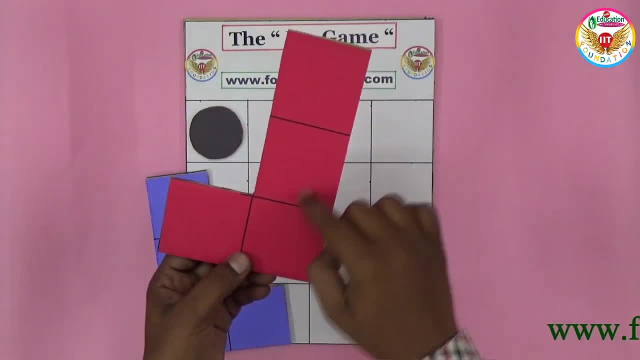 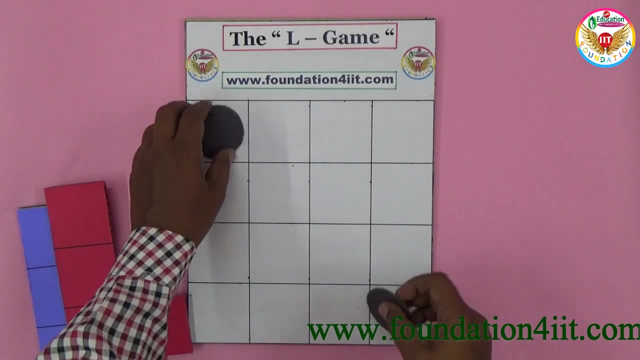 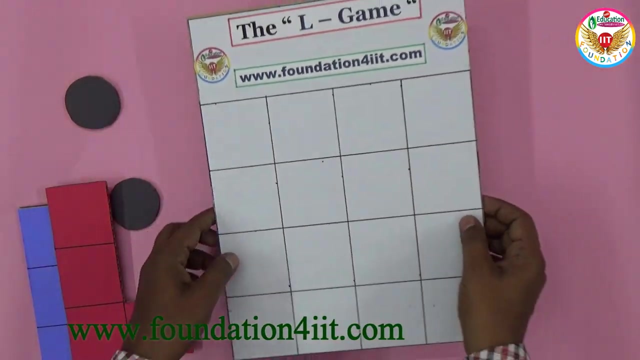 This is L shape. There are two L shape, Front side and back side same color. so one is red, one is blue we can use and two circular pieces. so just I use the cardboard for this and the model is this is a completely cardboard. I applied this is the four by four, so four rows and four columns, one cardboard. 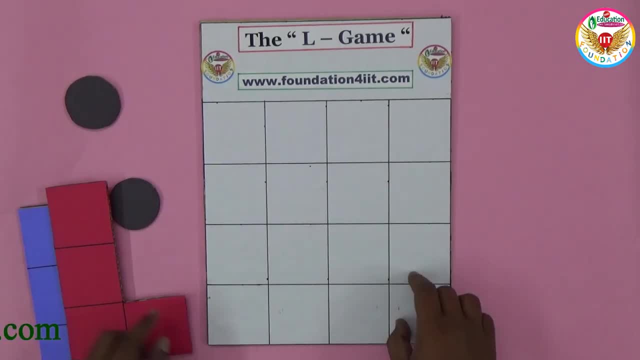 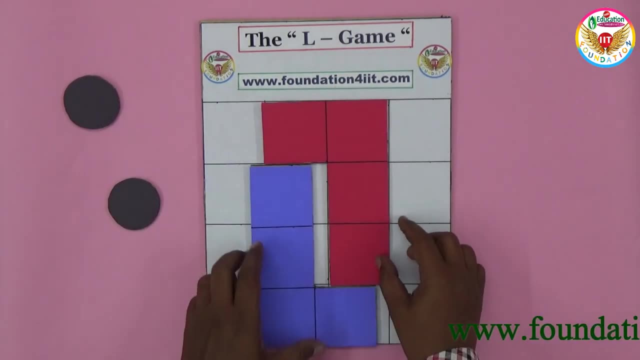 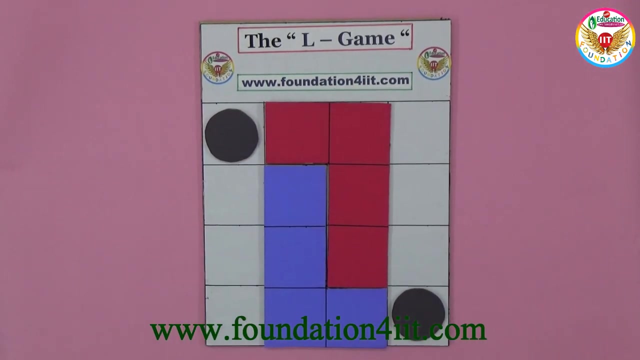 you should take and make equal length, so rows and columns should be equal length. so, after making this, yellow cards, so should keep the red like this, and blue in this way, and this two should be in this two corners, right, these two corners you should keep. now how to play this game and who will win. so this is: 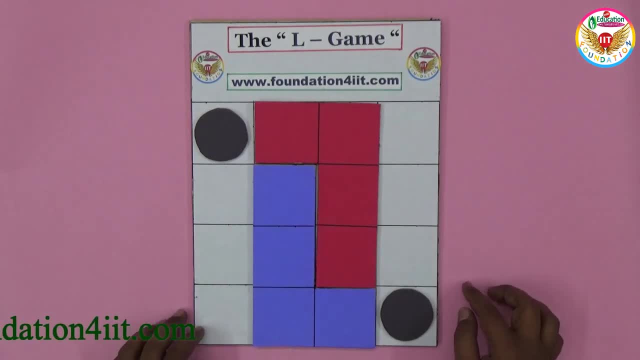 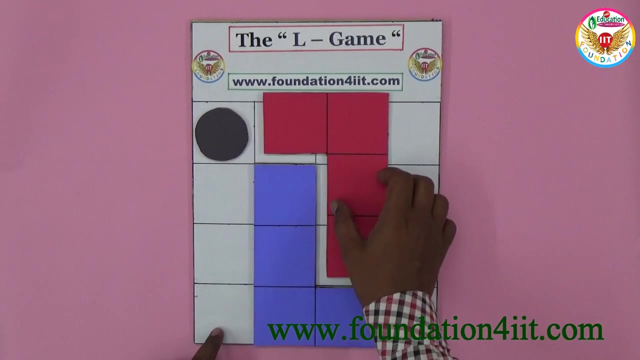 played by actually the two persons. so let us take A and B now, for example, A is playing with red card, red color and blue B it is playing with the blue. now this, for example: if you choose the A: A is playing with red. now you should lift up. 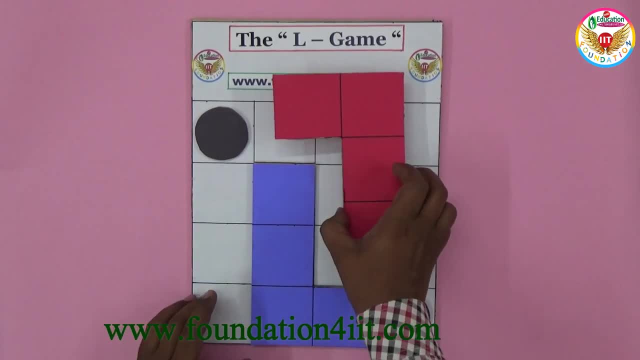 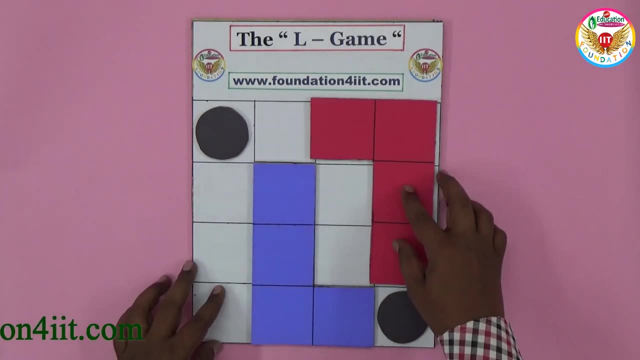 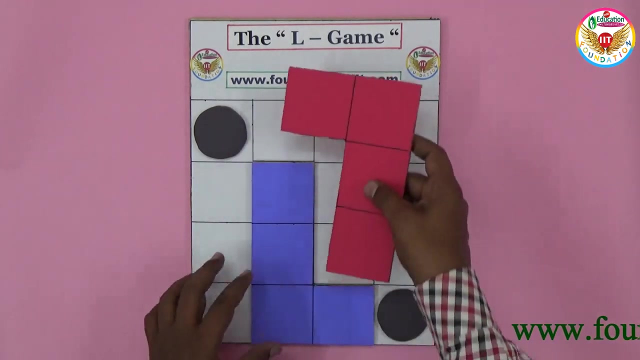 this is all right already positions, so you should remove this and should keep any other places. now, presently it is like this: we should change the place, so you can keep, even like this also, otherwise you can keep in this way. that means you should change this position. so previous is like this A position, so you should take out this and 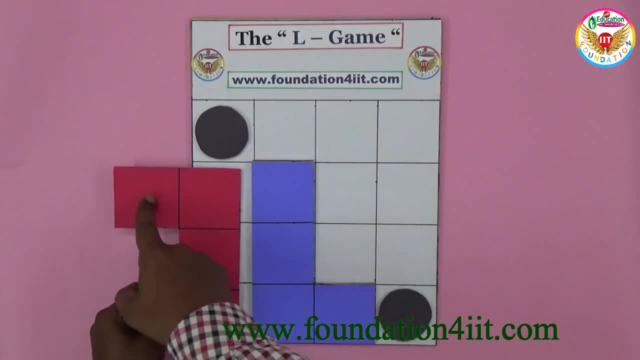 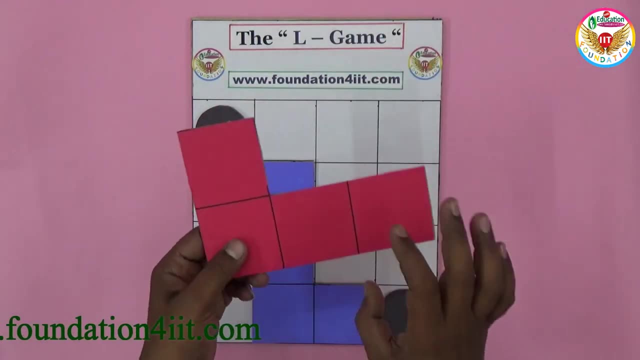 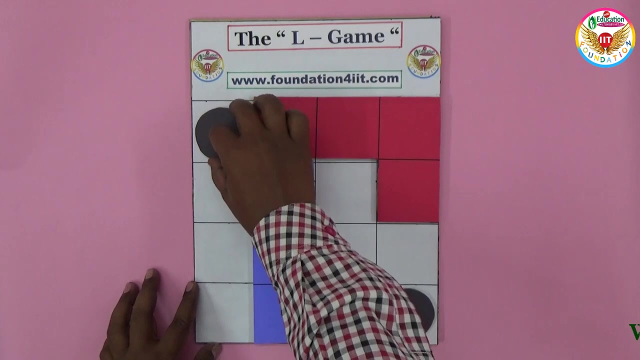 you should change another position. you can't keep like this because it's extra. so within the four by four box only you need to arrange this card. so previous it's here. now imagine, just to example: ok, kept in this way, he kept his changes card and one of this in this, both anyone. 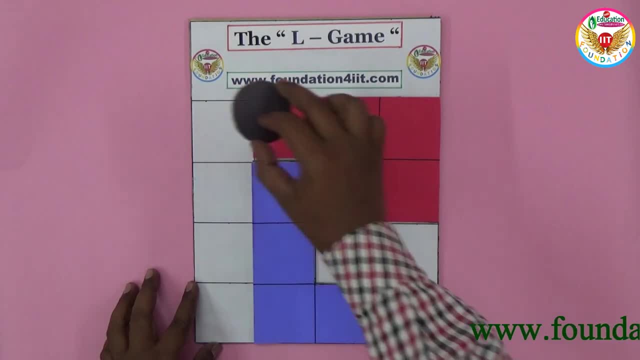 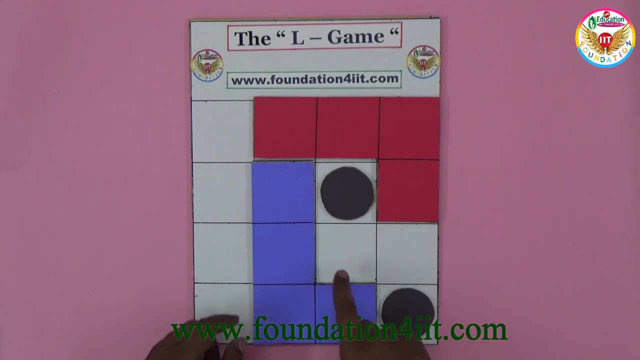 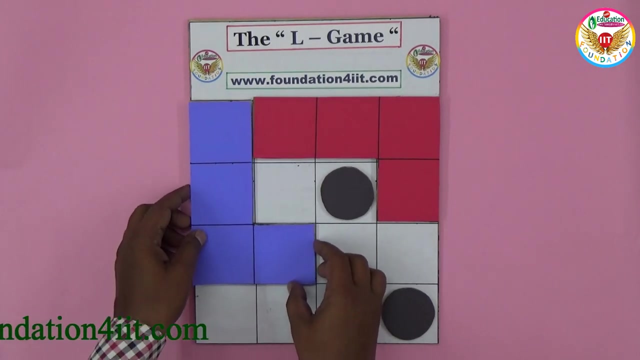 can change the position. ok now from here, imagine, just kept like this. now, next is blue turn, so this B. so player B is playing this blue, and if you can lift up you can keep any other place. for example, you can keep like this. now. the main condition is we should not give to opponent person chance. now blue can keep. 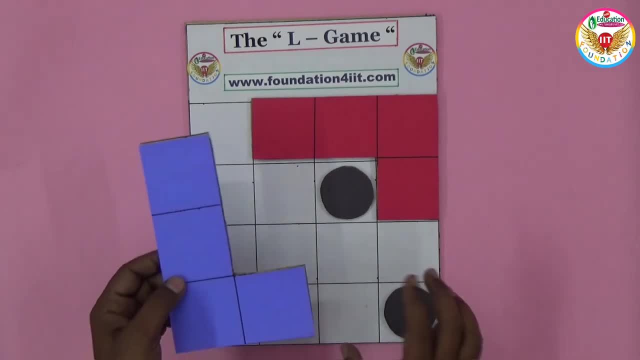 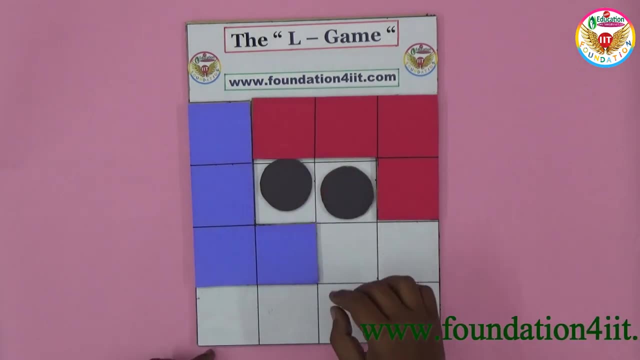 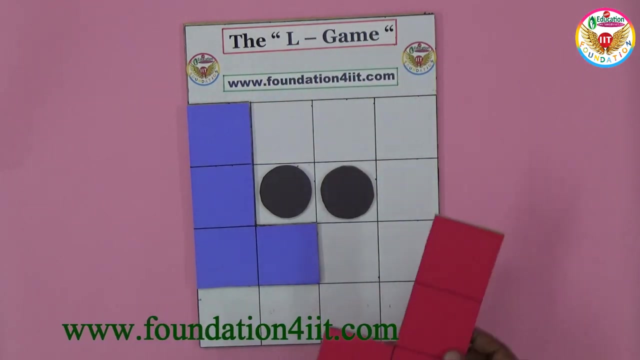 say: but if for this blue there is no, any chance means nothing. but the red who choose the red is a winner. now, blue, you can keep and is taking and keeping in this place. now the chance to the red so you can lift up, let him be- is keeping in.